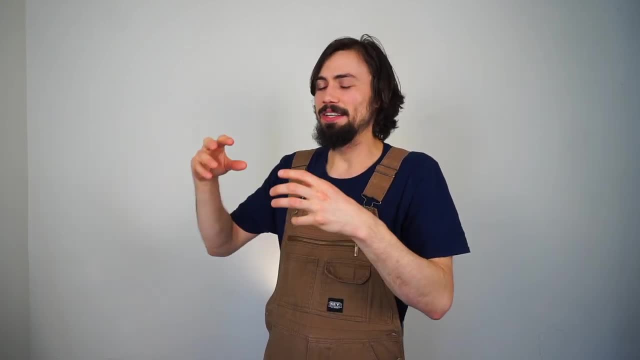 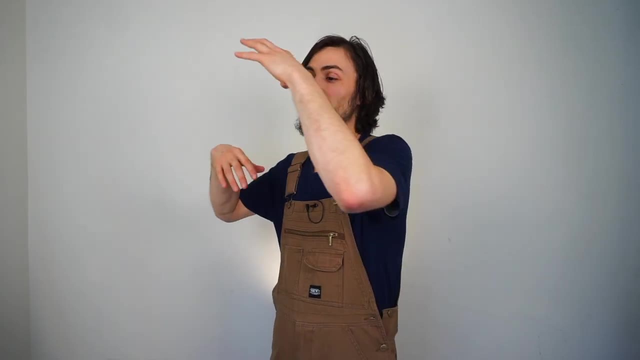 You want fungus that can attack those nematodes and eat them. You want, you know, you want the microarthropods to be shredding the fungi. You want the nematodes, the microarthropods and the protozoes all to be breaking down the organic matter too. You want it all to be continuously in a process of turning into humus, Turning into soluble nutrients. Bacteria will not break down your clays, sands and silts. That's going to be fungi's job. They're simple compounds. 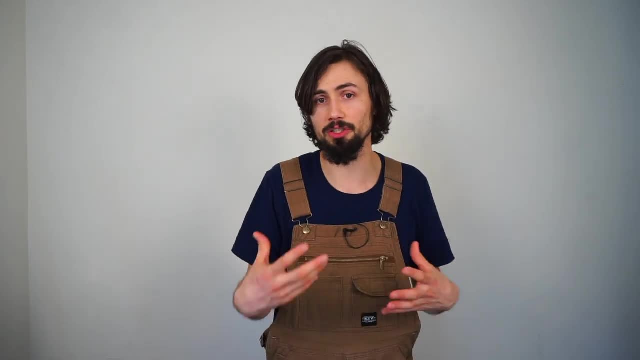 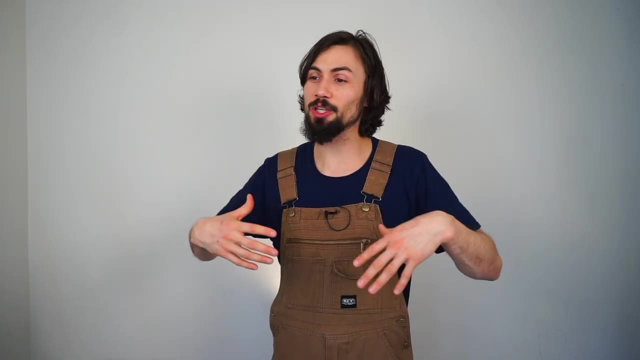 And yes, there's chitin and yes there's cellulose that can break down. There's special ones that can do that, We'll get into that later- But primarily bacteria is. they're the forerunners, They're going to go in and they're going to create those glues to make the microaggregates. 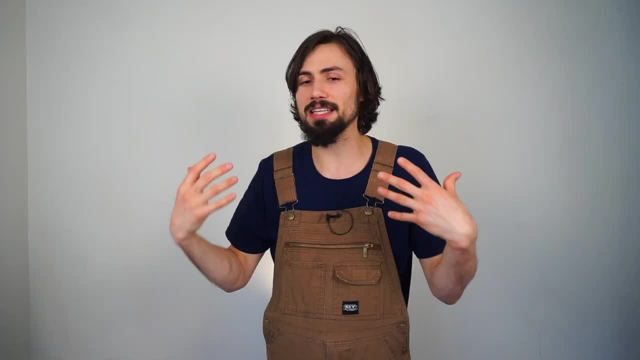 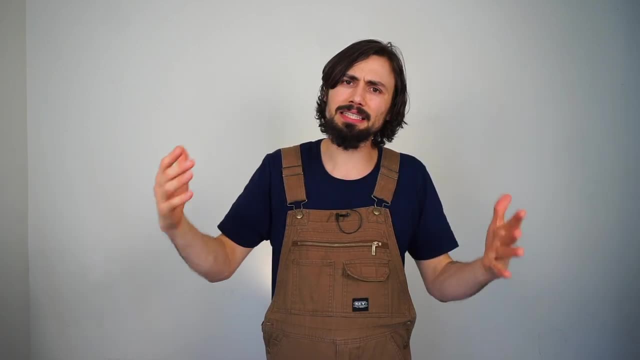 for the macroaggregates to be put together by fungi. They're going to set the stage. Their populations actually don't decline as we travel in succession. They basically stay stable, They set up shop and they're there When they're overpopulated. that's when you have problems. 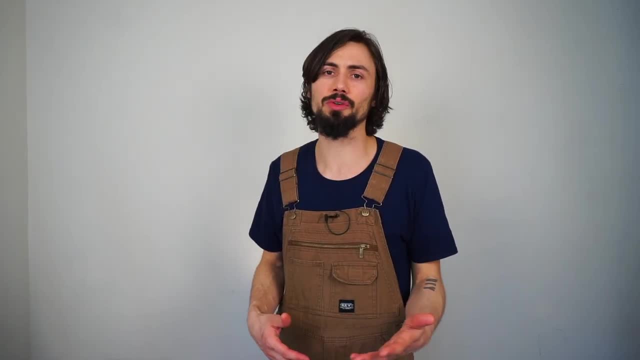 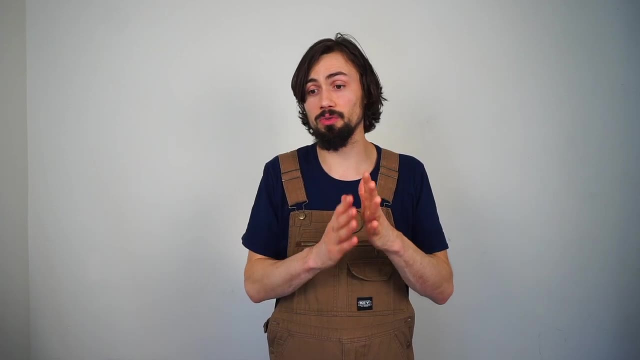 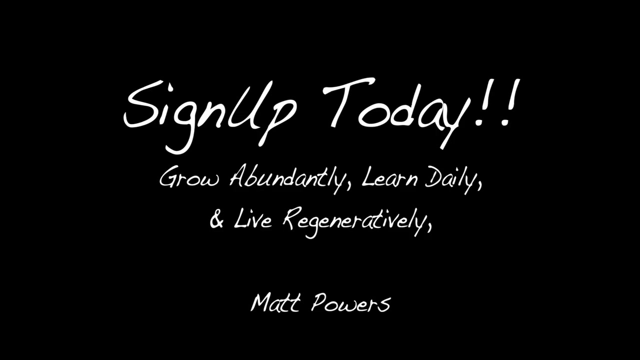 Bacterial dominated soils are the ones that are the nitrate dominated soils, which are the weedy soils. So if it's all just bacteria, if it's tilled and you destroy all the fungi, then you've got just bacteria left. What is the best way to deal with that? 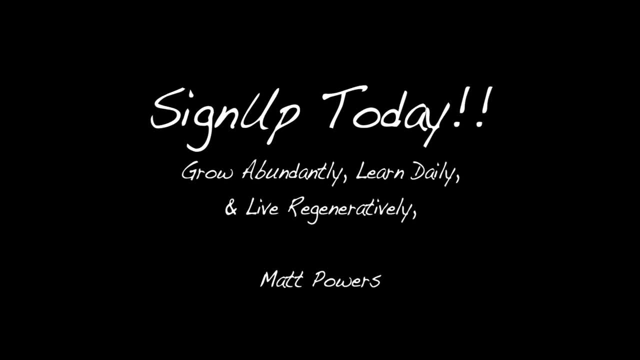 No, but if that's the case, there's nothing much we can do. We can't go out and buy a disease and then consume it. We can't go out and buy a plant that doesn't have any pesticides. We can't go out and buy a plant that has a pesticide. If the ones that are going to die are pure beetles or other food types, then we've got to help them. I just want to make sure that everybody's heard that testimony And I can't tell you when you get to that point. I'm just going to ask you to let me know. let me know if it's a good thing for you and I can let you know if it's a bad thing for you. That's what I'm saying. That's good, Thank you. Thank you. 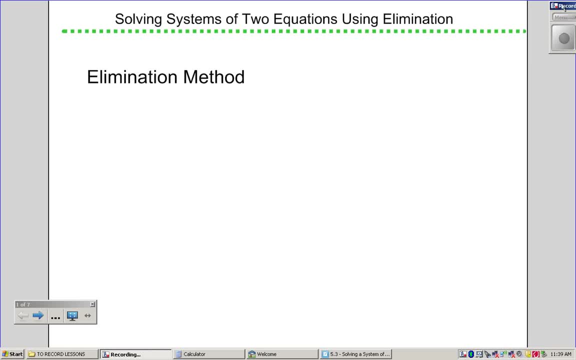 Hello and welcome to today's lesson, Lesson 5.3, Solving a System of Equations by Elimination. In our previous two lessons we've solved system of equations by graphing and by using the substitution method. Today we're going to learn about the elimination method. 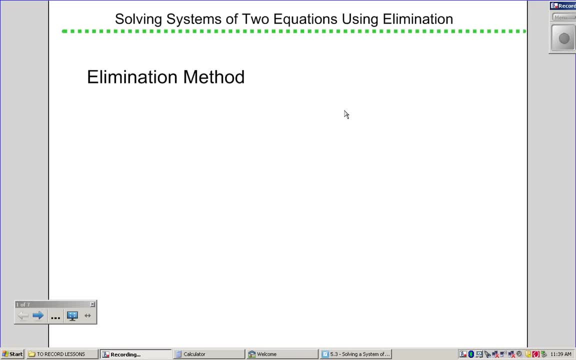 Elimination method, basically, is telling us that we're going to eliminate one of the variables. So we're going to notice a relationship in our equations and it will allow us to eliminate or get rid of one of the variables that we are set up with or starting with. 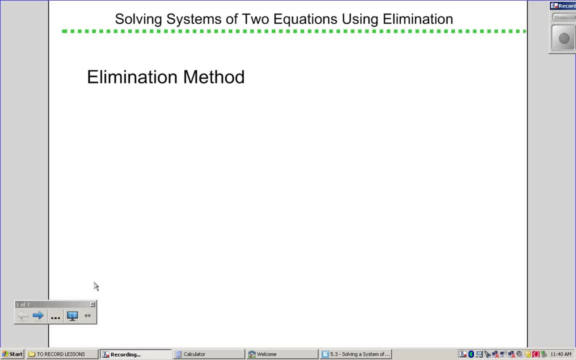 So let's take a look here at our first example, and we'll just dive right in. So, as I'm solving the system, I'm going to be using elimination. So you'll notice that there's not one variable written for itself. It's not written in slope intercept form.